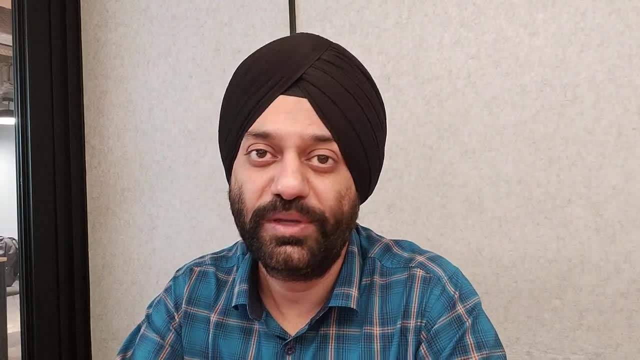 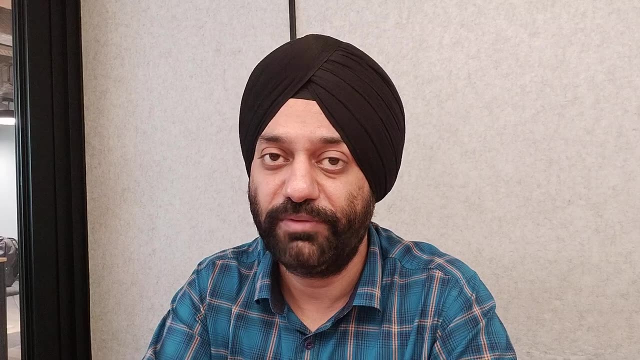 think this happens in sentence correction and quant. These two are similar sections. Let's say you're solving a sentence correction question and you have already done all the theory part, because I'm talking about people you have already given GMAT, So I assume that they have been through the all the. 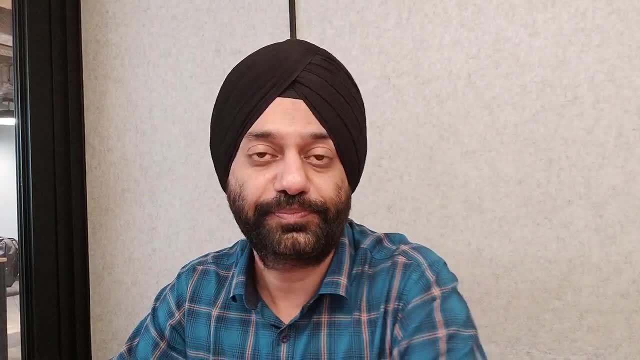 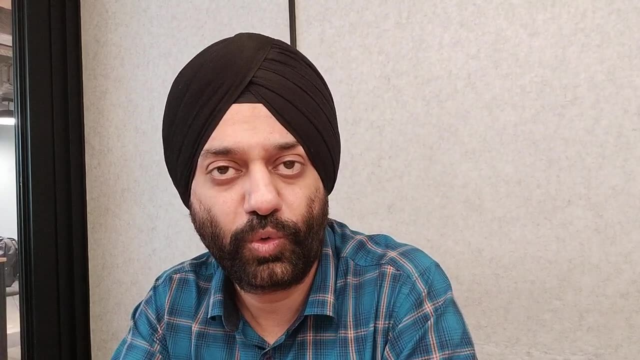 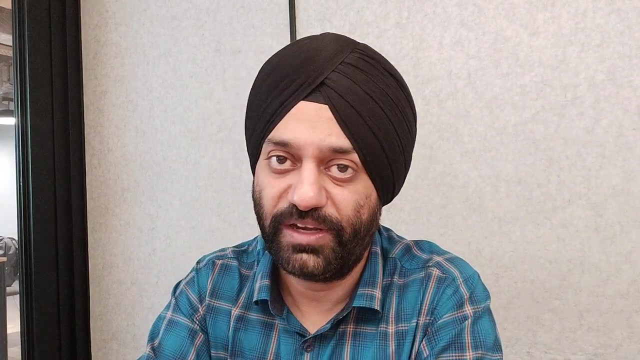 theory part, but still they are getting the questions wrong. So what happens when they practice? So let's say they are solving a sentence correction question and it's around 650, 700 level question. So when they solve the question, if the question is based on the topic in which they are comfortable with, 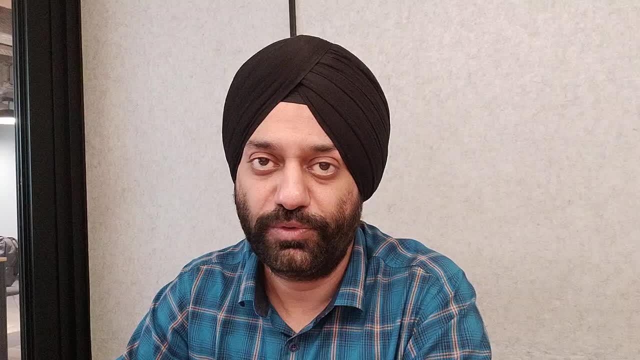 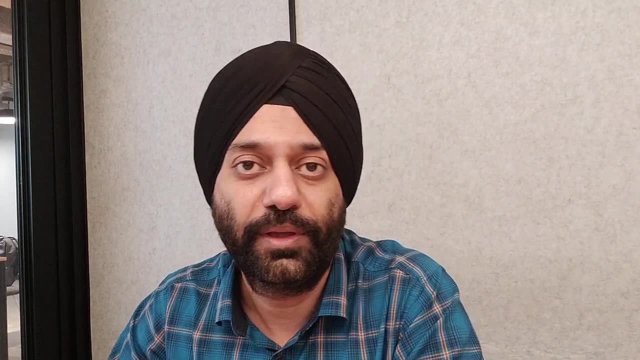 let's say it's a singular plural verb error, so they will be able to solve that question. It's a 600, 650, 700 level, but it's on singular plural verb, so they will be able to solve it. But if the topic is: 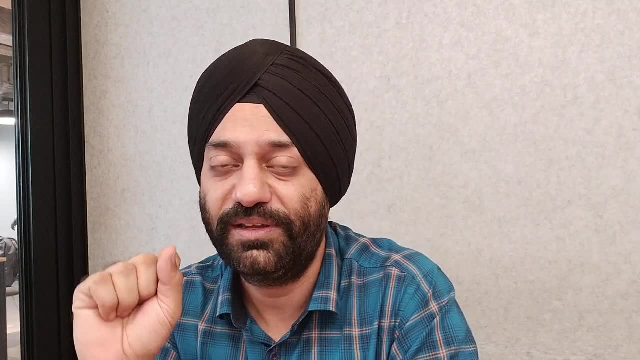 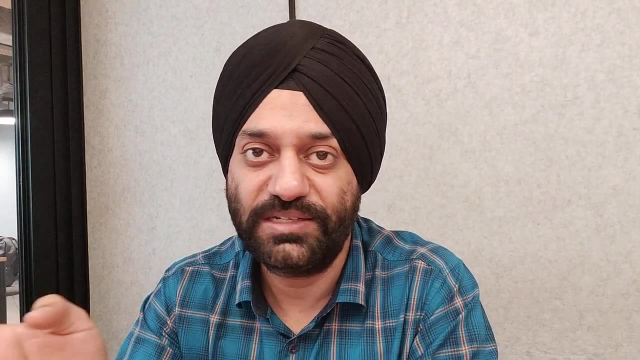 let's say it's tensed and you are aware of the theory, but you are not comfortable with tenses. and this is what i have seen: that most of the students are not comfortable with tenses, specifically present perfect tense and past perfect tense. so let's say you're solving. 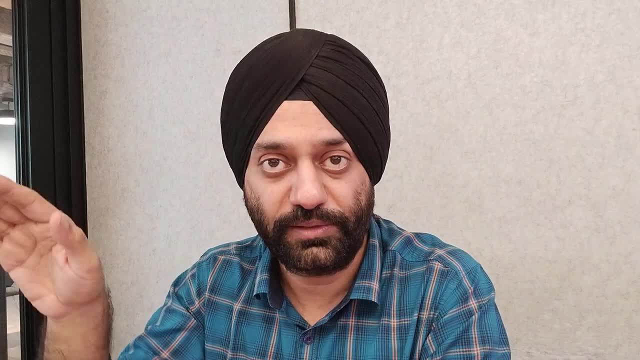 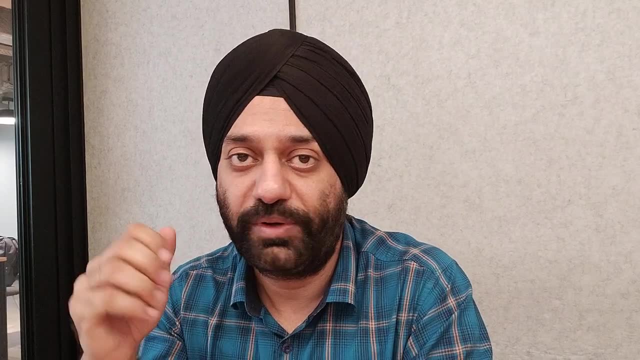 the question and you see the tense error. but mostly what they do, they ignore it. so ignore that error and just looking for the errors that they are comfortable with. but that error is not present and that's a tense based question. so the one thing that they normally 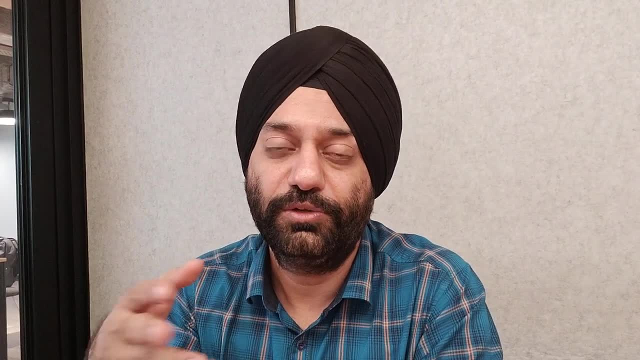 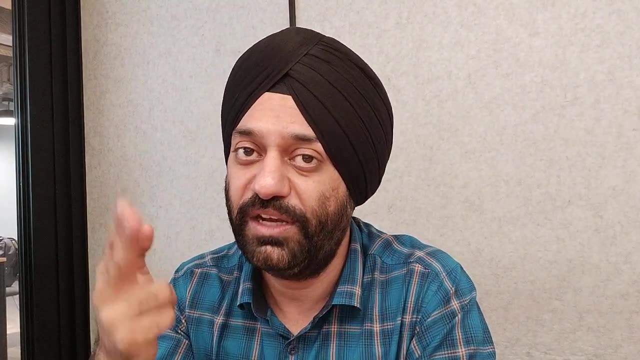 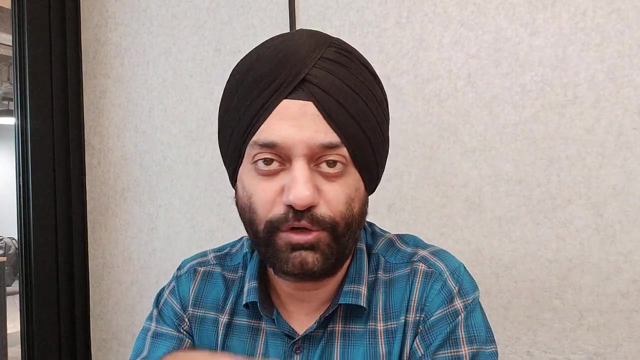 do. is that okay? they, because they have to somehow give the answer, so they simply just start reading the sentence, read the options and just work on their intuitions and, based on their intuitions, they take the decision. and once they they are done with the question and they know they got. 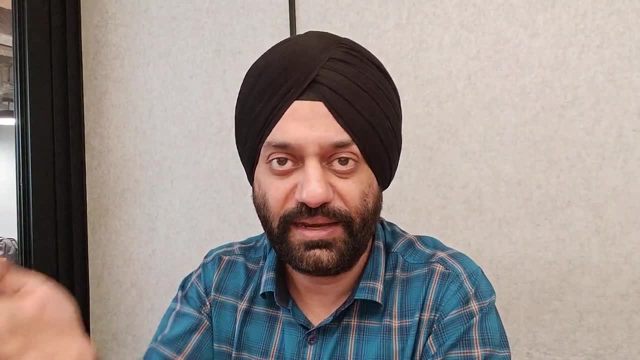 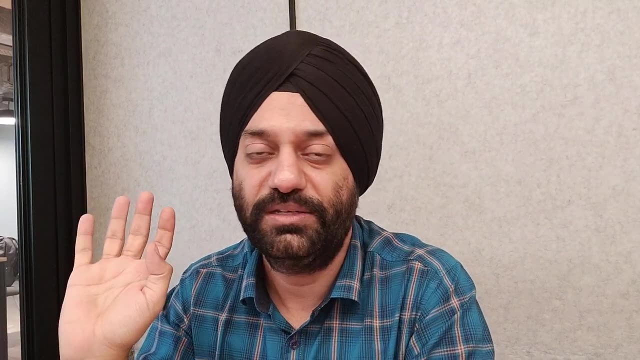 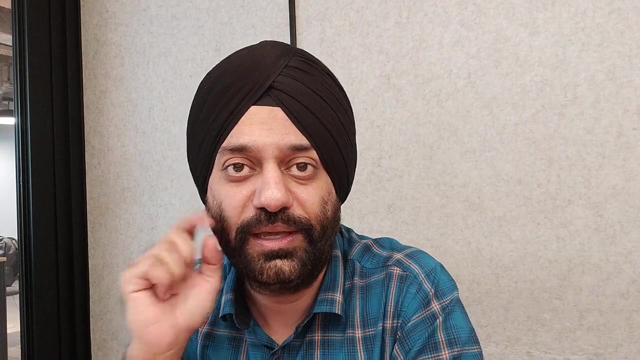 they got that question wrong, they go to the gmat club and they start reading the explanations given at the below the question and when they read the explanation they think, okay, now i understand that, but next time when they get the same question on the same topic, they get it wrong. this is where everybody 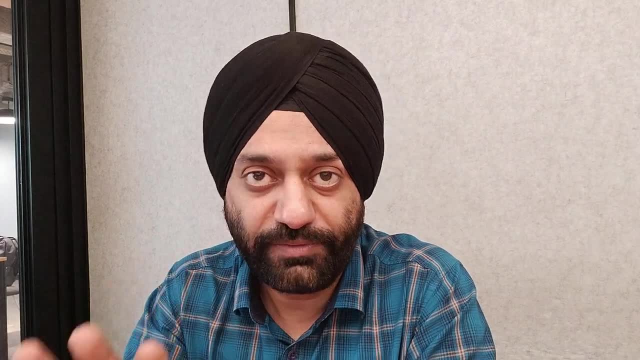 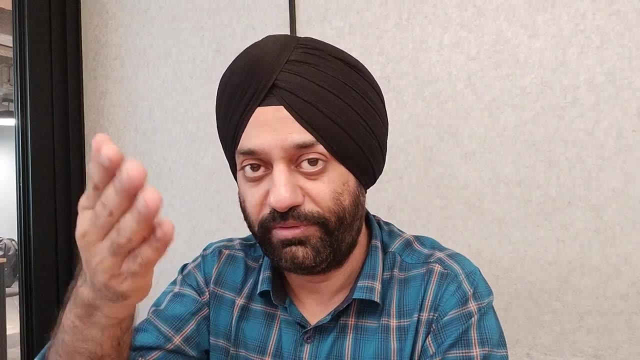 who is in this range is stuck. what you have to do is that, let's say, you get the question wrong and you know that it's a tense question. the other thing that normally do is: you know one thing is that you read the explanation. second is that you know they just doubt themselves and they go back. 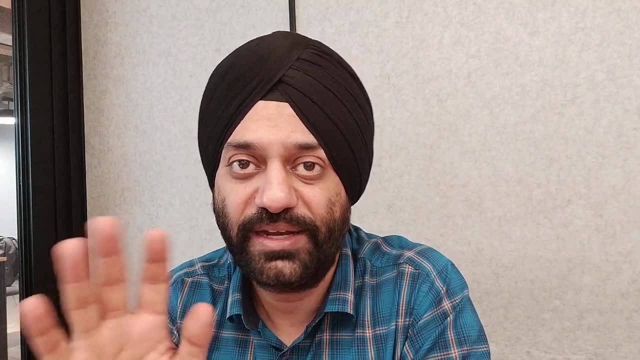 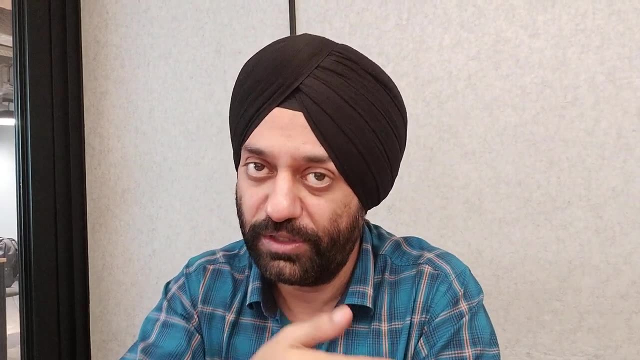 and revise their entire theory. these are the only two things that everyone is doing, nothing else. when you get the same question on the same topic, you get the same question on the same topic and you get the question wrong. okay, i'm assuming that because you have read all the theory only. 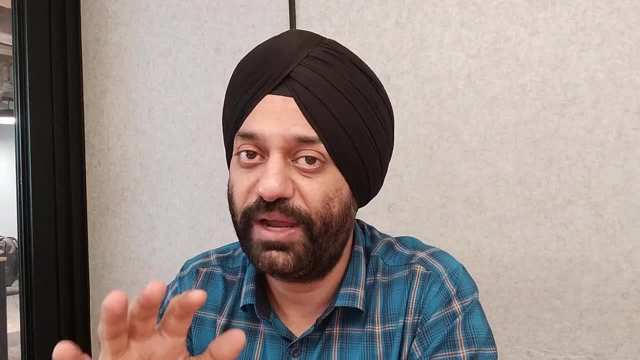 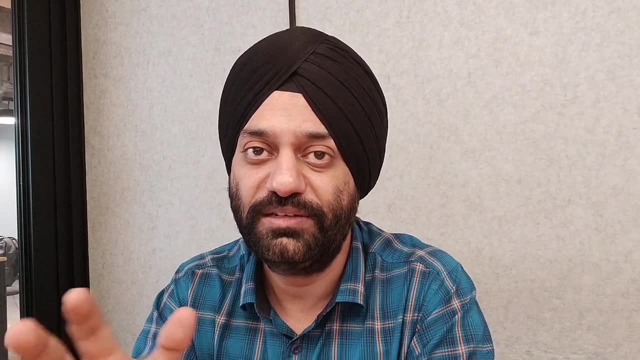 that you are attempting 650- 700 level question. that means you don't have to go back to the theory. the only thing is you don't know how to use that theory. how do you use that? okay, let's say the question is on past perfect tense. so when you're solving a sentence, correction question, so you 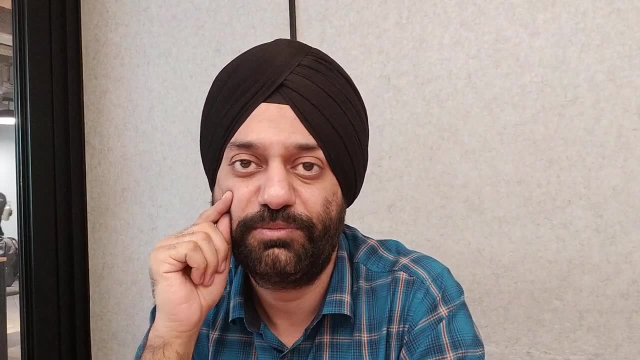 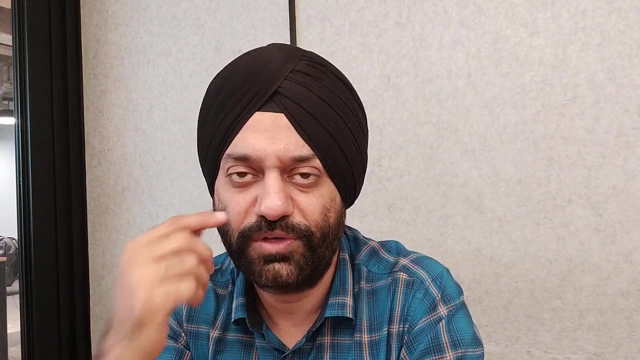 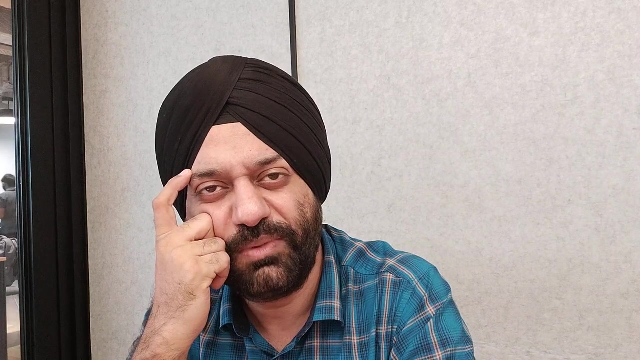 saw a past perfect in two options and three options. we don't have past perfect. that means past perfect is correct or past perfect is wrong. so i was most of the when. you know, i'm discussing a question with the students, so i just ask them: do you know, uh, how past perfect tense is used? uh, i know the theory but you know, i don't remember. 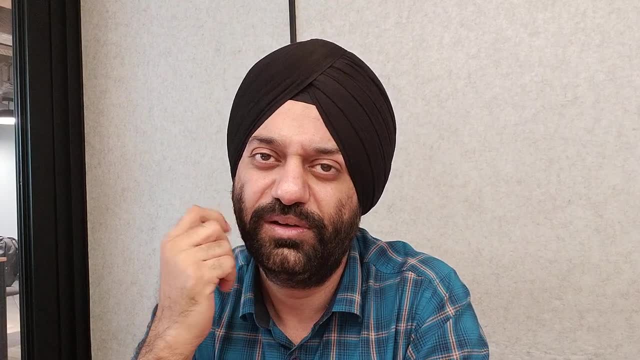 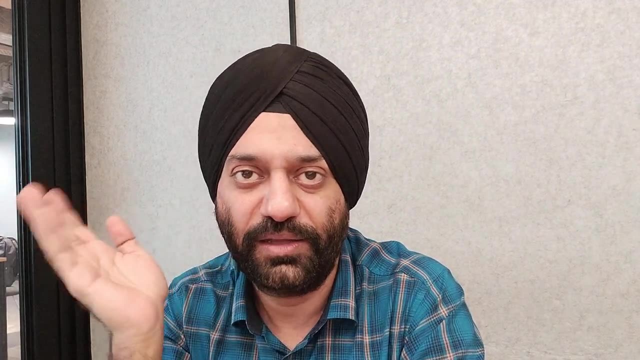 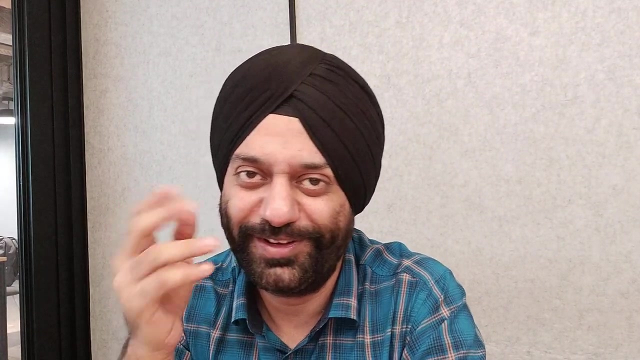 the usage. so i ask them: okay, tell me the theory. uh, it's something in the past i don't remember exactly. i ask them: you don't remember it or you don't want to go back, and you know, ask yourself exactly what it means. i say: what does it mean? okay, to explain this, okay. 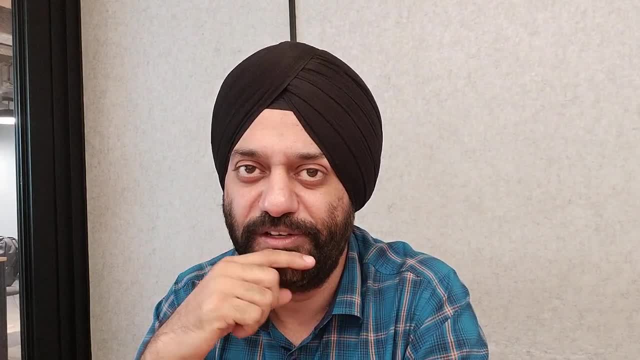 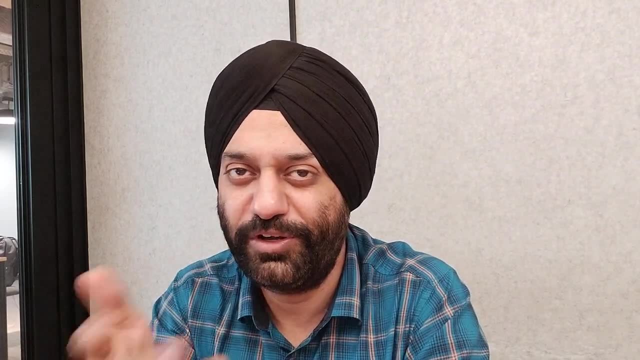 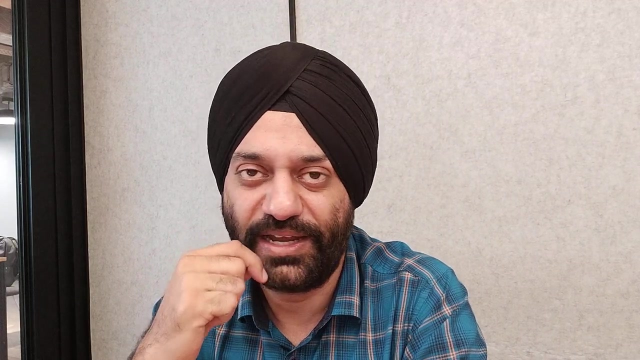 i tell them: okay, uh, have you had? did you have your breakfast? he said. the person says yes, okay, i asked them what did you have in the breakfast? so they let's say bread, omelet. okay, great, you remember. then i asked them: did you have your dinner last night? so they say yes, 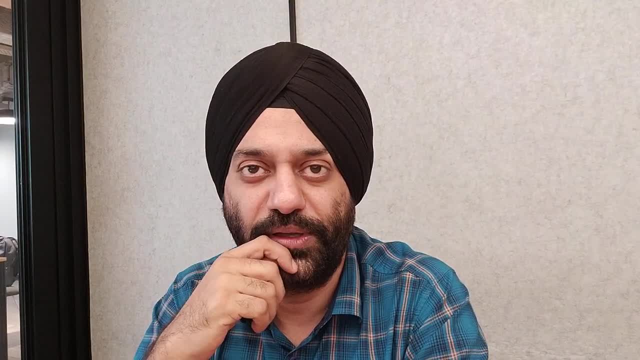 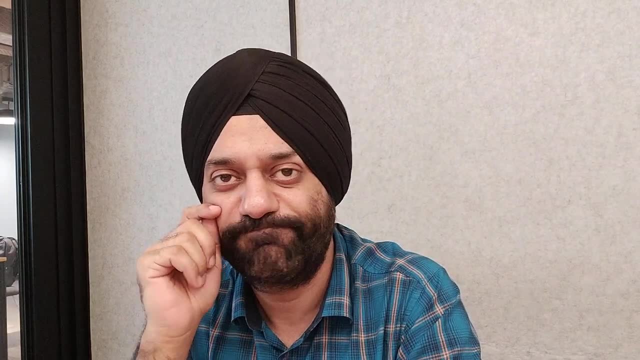 so i asked them: do you remember? most of them do. then i asked them: uh, let's say, today is 31st march. so i asked them: do you remember what you ate on 15th march? and lunch? i don't know. okay, so can i say: can you go back to your memory lane and tell me, or you don't know? 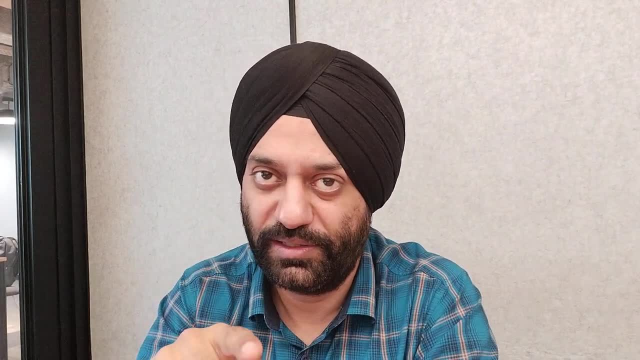 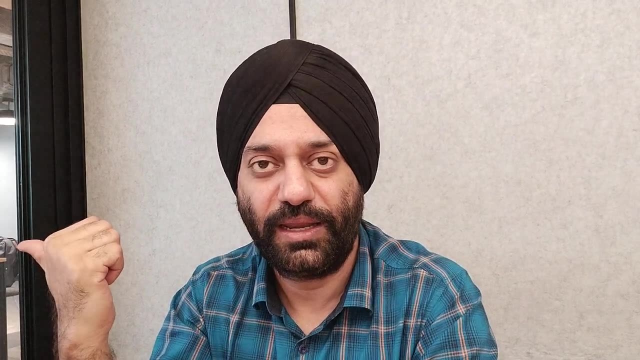 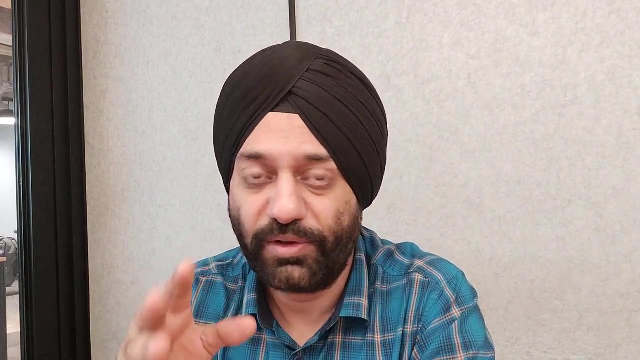 because you ate and if you have done something it will be part of your memory. but you don't want to go back to the memory lane and think this is the problem with maximum students: they don't want to think. thinking is that okay? ask them if you have to tell me, okay. 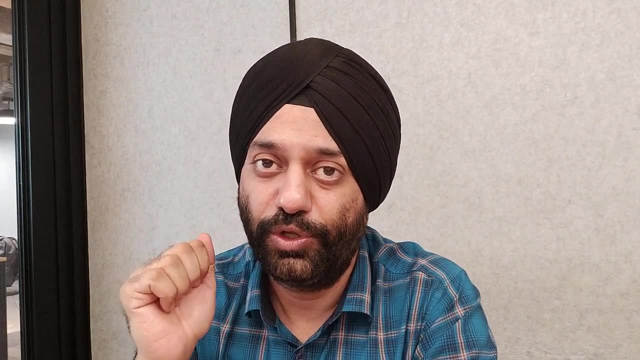 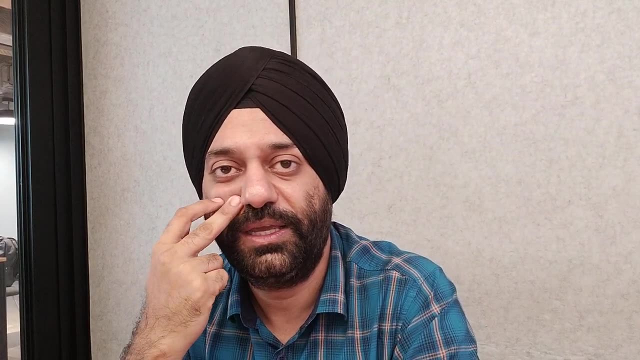 what you ate on 15th march in your lunch. so what will you do? so he says, okay, i have to think: okay, what day was it? so let's say 31st march is sunday, so you just go back. okay, minus 7 is 24. 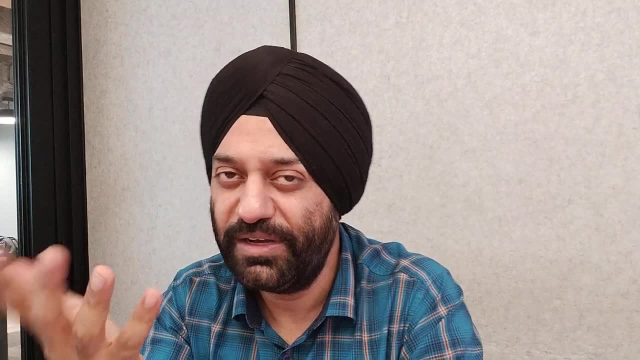 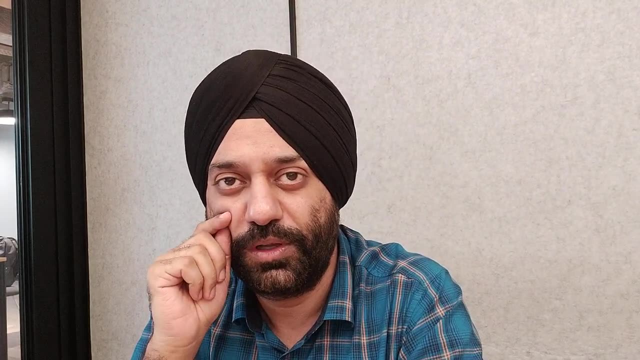 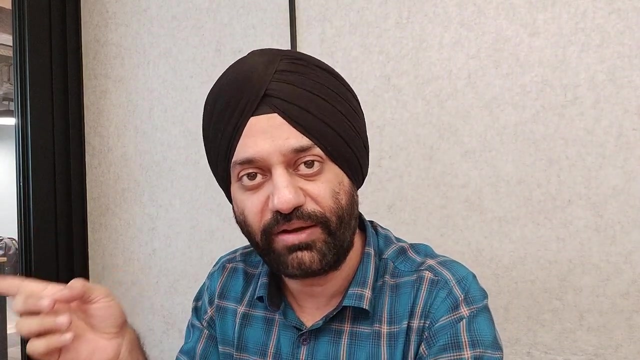 so minus 7 is 17, so probably it would be friday and then uh, on friday would normally i was in office or i was at home. if i was at office, what normally do i eat in the lunch? are you saying i'm asking right questions to reach that right answer. let's say the person ate uh pasta on friday on. 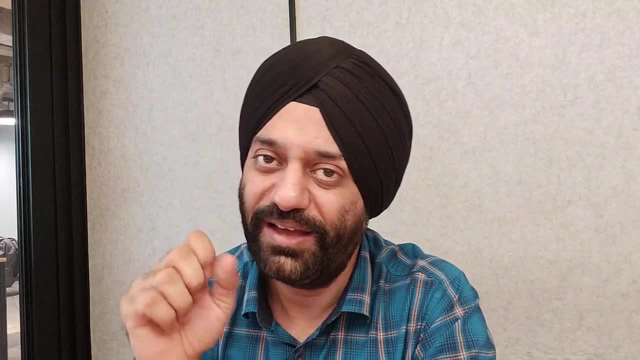 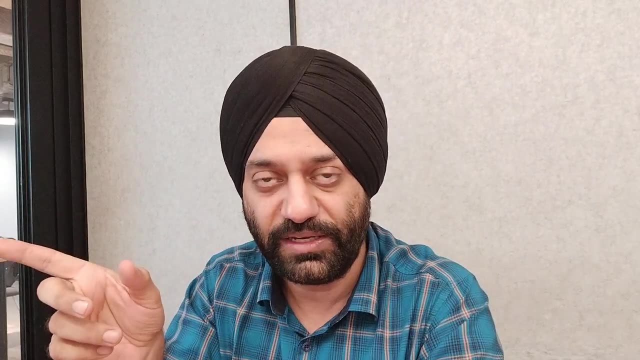 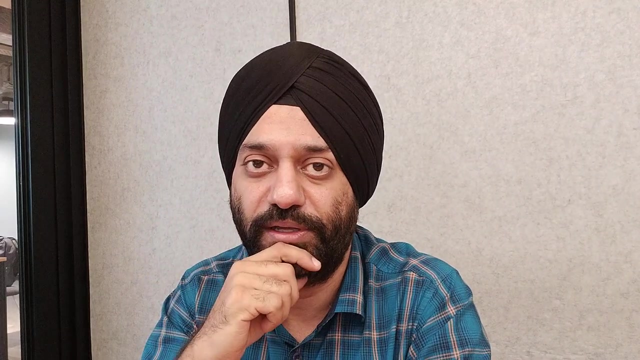 15th march in lunch. i asked them if i asked the same question that what you ate on 15th march in lunch, probably after a week, will you take the same amount of time or you will take less time? he said: i'll take less time. it's just the same thing. happens in the sentence. correction and quote. 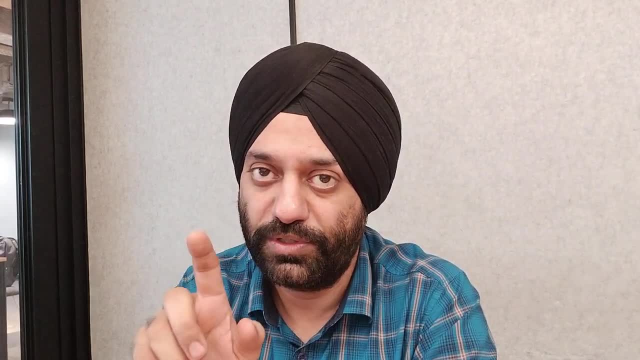 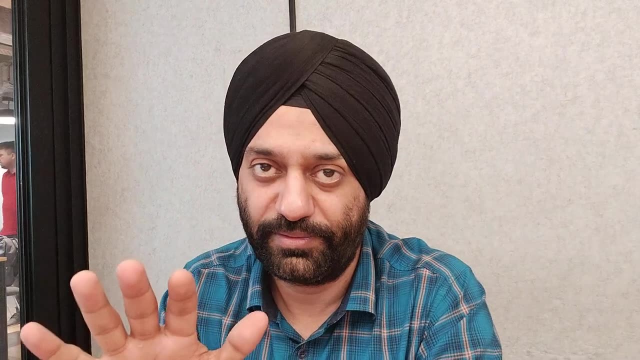 when you're practicing and if you are stuck at a question, you have to go back to your memory lane and ask: how do we use past perfect tense? and you have to stay there. okay, may it take five minutes, minutes, 10 minutes, 15 minutes, 20 minutes, half an hour. I've never seen a student giving. 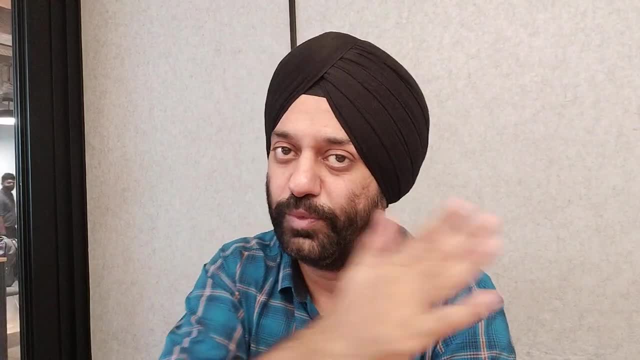 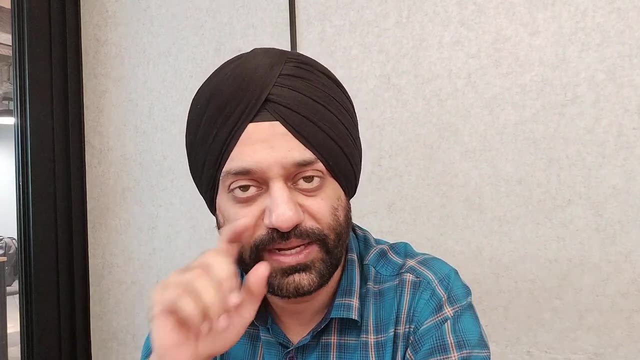 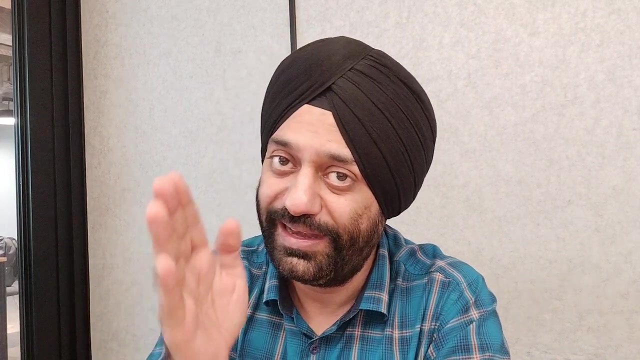 more than probably 2 to 3 minutes on a particular error. They switch. They are not able to think through on a particular error. So if you just you know when you're practicing and you just sit with that quotient and you handle that past perfect tense yourself Once it's done, 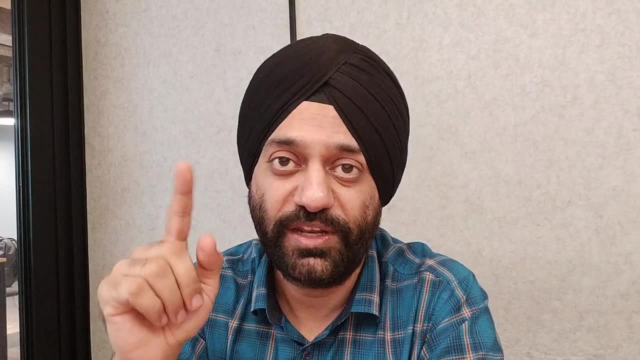 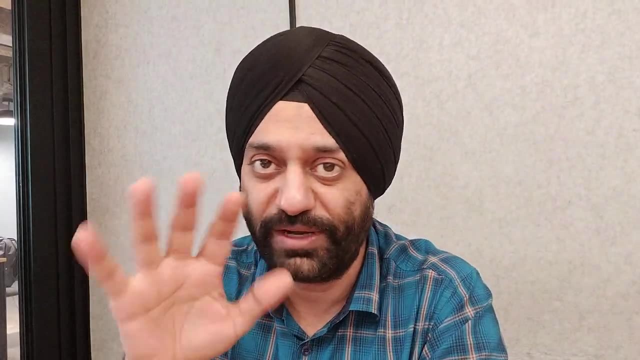 next time, if you get the same quotient and the same error, you can solve it in a minutes time. This is what happens, And if you're not doing this with every error- because there are limited errors, it's not infinite. There are finite number of errors in SC and CONT. 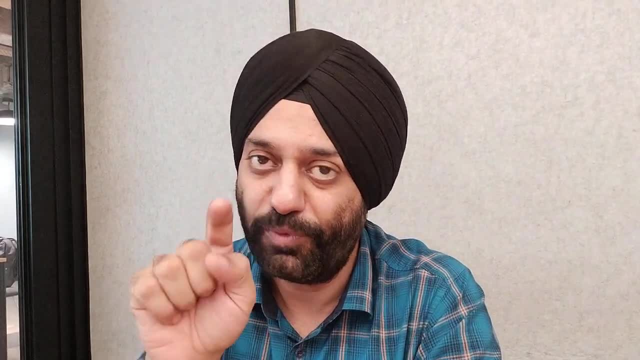 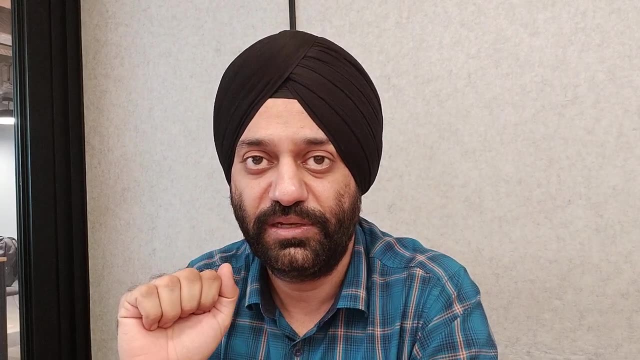 because these are two similar topics which are based on theory. If you approach this way and you just give time in your practice and trust me, it will take only a month's time to master SC. but you give almost a year because you don't go and think. If you master, 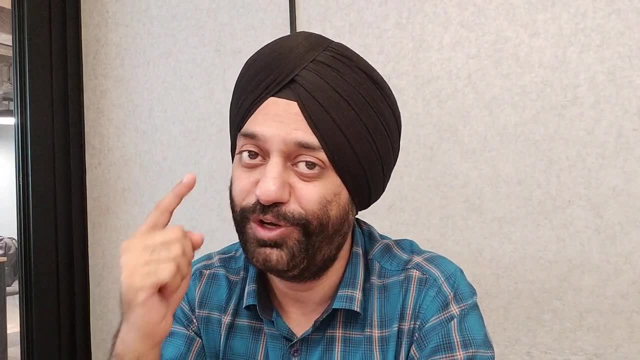 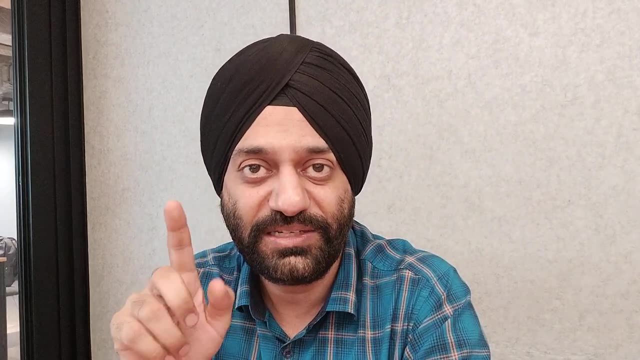 this one mindset, you will see immediate improvement. And if you're not doing this, irrespective what you do, you do thousands of quotients. you're not going anywhere. You're here, So try this out and see. is it helping you, or? not, Thank you.